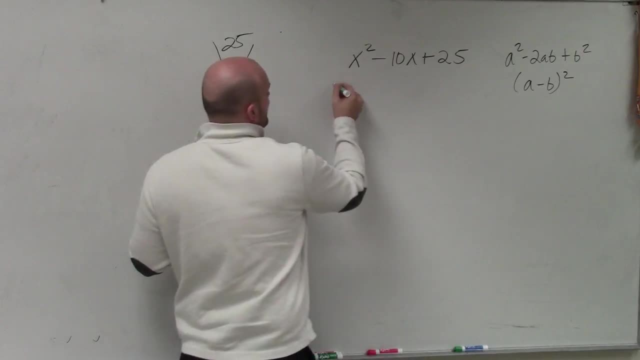 So let's double check this. So let's figure out what is the square root of our. so if a squared is a squared term and b squared is a squared term, let's figure out what a and b is, so I can easily plug it into that format. 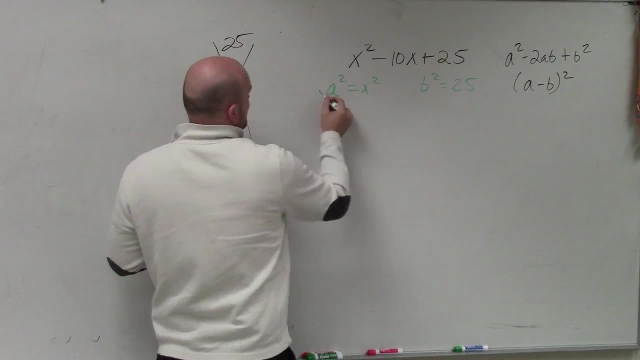 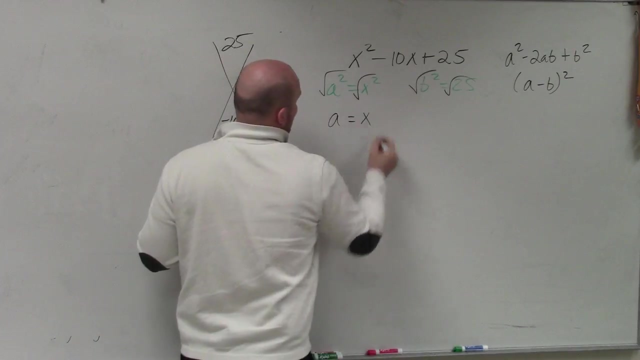 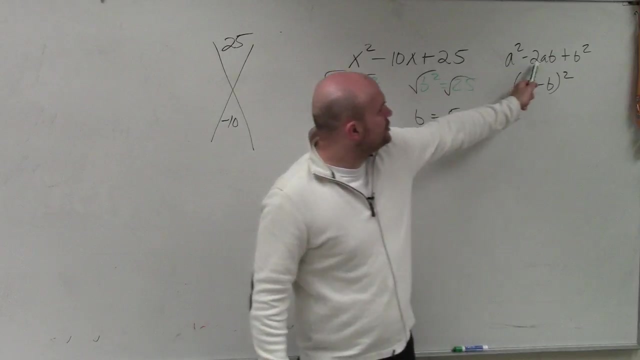 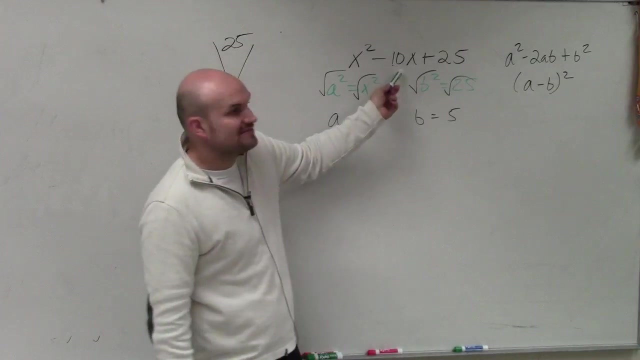 So what I do is I take the square root of both of them and I get a equals x and b equals 5.. Would everybody agree with me? Now is my middle term? 2 times a times b. 2 times a is x times b. What times 5 would be 10x, right? Do I have 10x there? 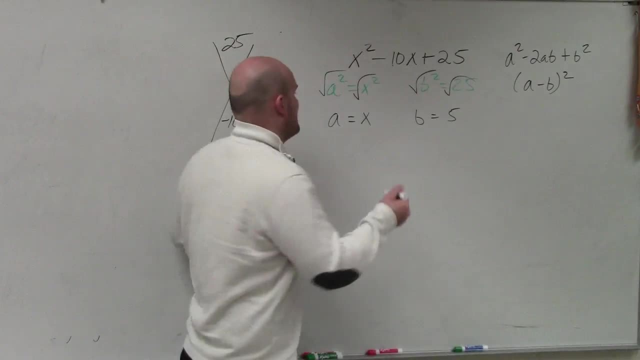 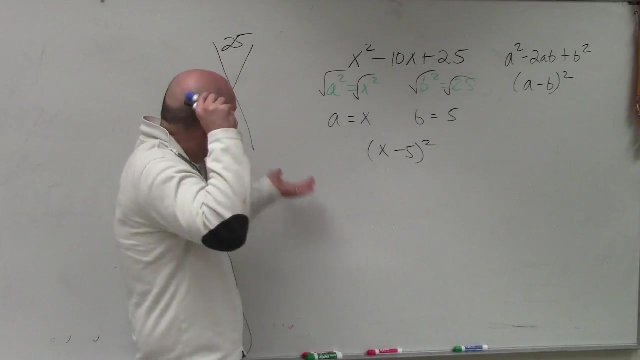 Yes, And since that's subtraction, that's subtraction. So therefore, my factored form is just going to be x minus 5 squared. Okay, Now you might say, Mr McLogan, I already knew that was going to be negative 5, right, That's easy. Why would I go through that when I already know? 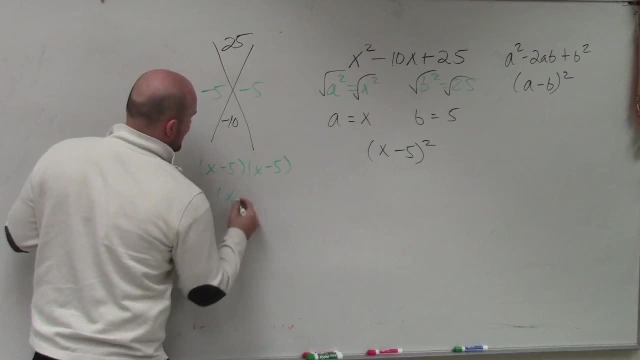 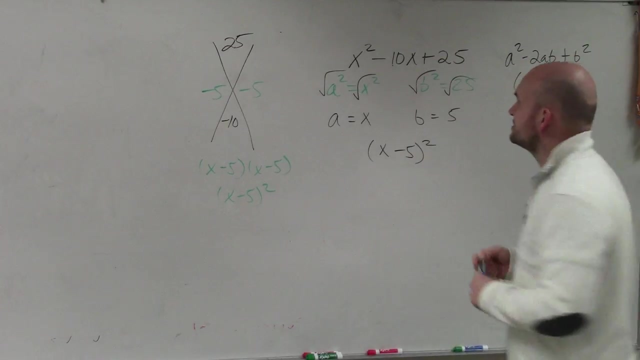 that it's x minus 5 times x minus 5, which is x minus 5 squared. I like using the trinomial method. I'd rather just use that, right, It makes sense. Why would we do this? Well, because of the. 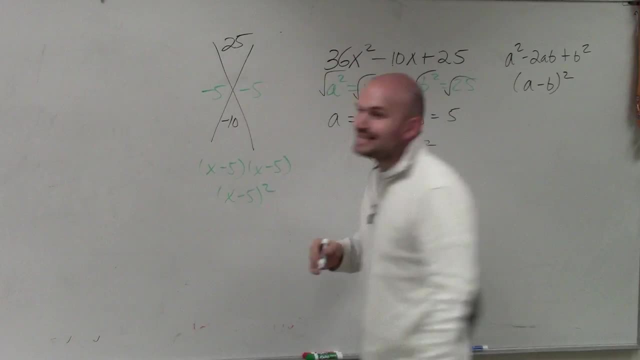 same fact. ladies and gentlemen, what if I made the problem like that? What if it was 36x squared? All right, If it was 36x squared, are you going to want to do 36 times 25 and then figure out which one of those add up to give you negative 10?? 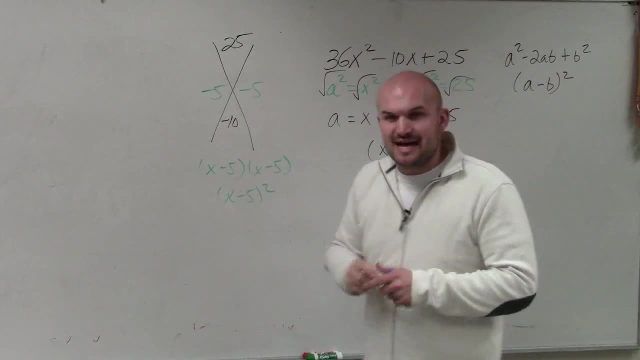 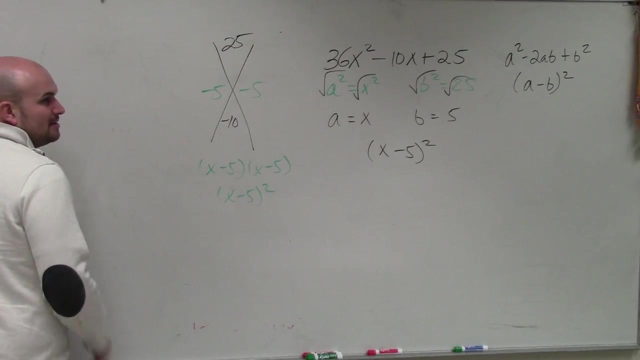 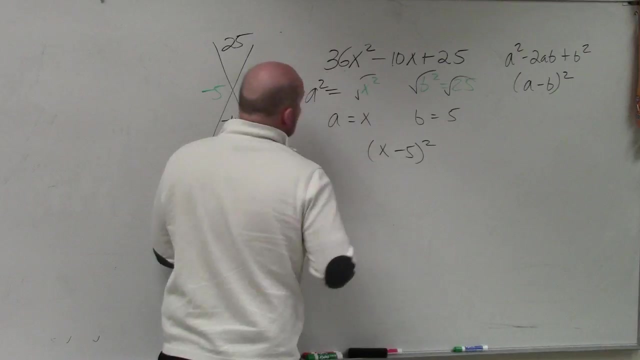 No, right? Well, first of all, our middle term has to change, But anyways, that could be a very difficult problem to do. However, is 36a squared a squared term? Yeah, Yeah, So I'd have: a squared equals 36.. 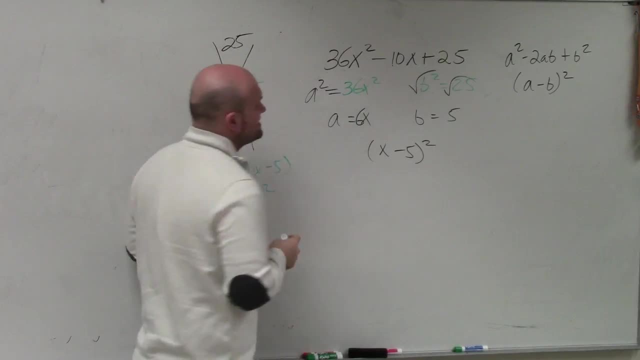 36a squared. So therefore, that would be 6x. Now, obviously, for this problem to be correct, I'd have to do 2 times this, which would be 60x. Okay, However, b would remain the same. 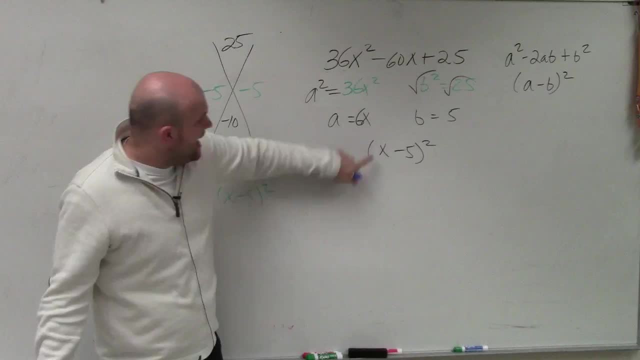 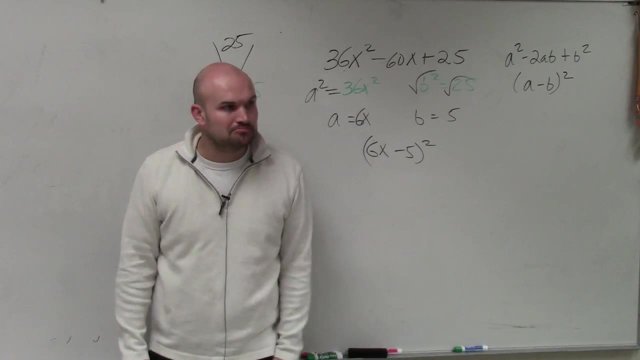 I would just take the square root of my first term and guess what Now? a is 6x, b is 5.. Boom, See how easy that was to factor. that Done, Okay. So if you have your first term as a square term,